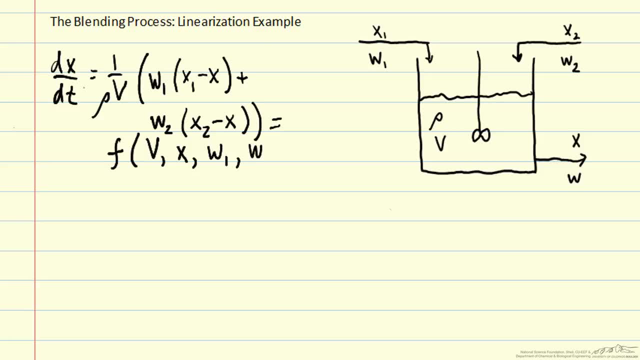 We also have inlet mass flow rates, w1 and w2.. And in this case we're going to assume that the mass fraction x is the mass fraction of the tank, That our density rho is constant. We're also going to assume that the inlet mass fractions x1 and x2 are constant. for this example, 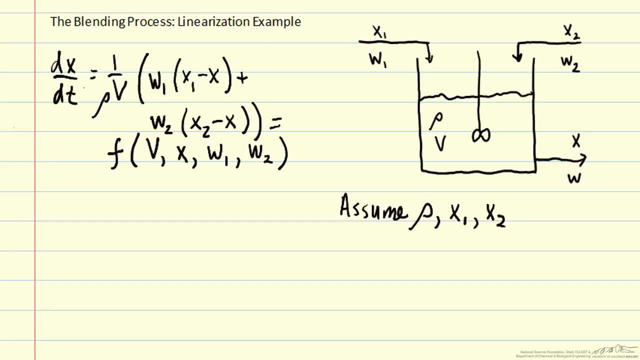 And now we're going to calculate the linearization of this nonlinear dynamic equation. For the left-hand side we'll substitute in deviation variables, So instead of x we'll have x bar the steady state value, plus x prime, the deviation from steady state. 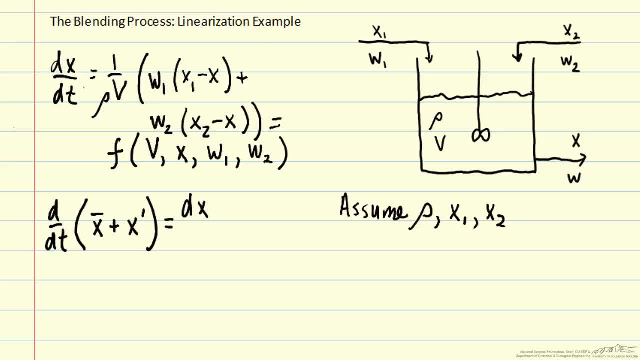 And because x bar is a constant, we can then simplify that to dx, prime, dt. So the deviation is time-varying but the steady state value is a constant. And then we're going to approximate the right-hand side by a first-order Taylor series approximation. 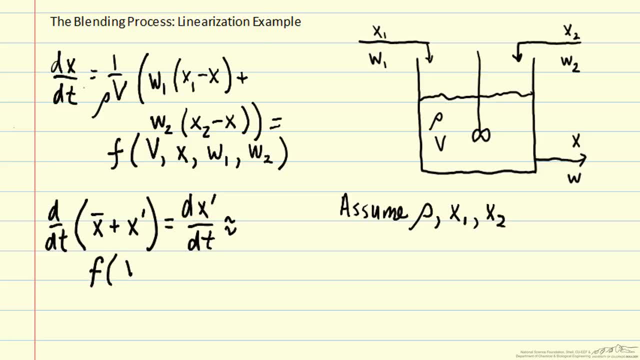 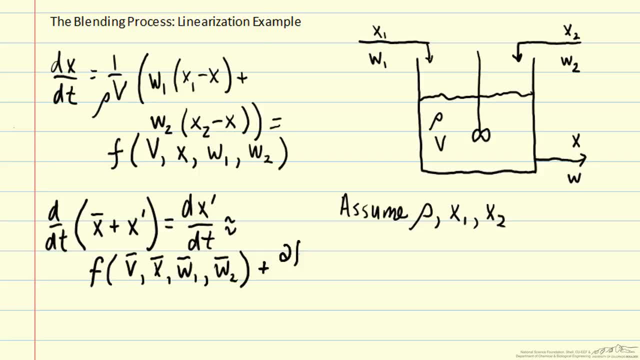 And our final term is f. So we have df dv evaluated at steady state. We'll use ss for steady state Times v prime plus df dx evaluated at steady state times s prime plus df dw 1, evaluated at steady state times: w1 prime. 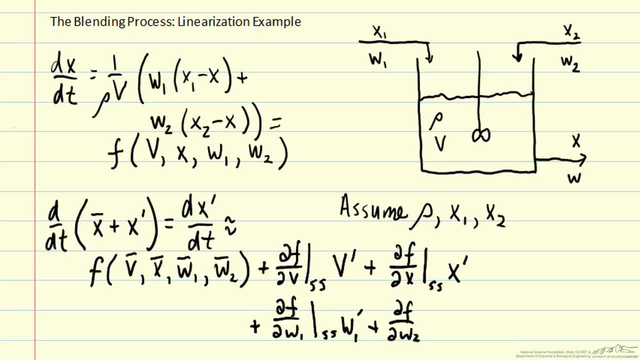 We'll use ss for steady state times- w1 prime. We'll use ss for steady state times- w1 prime. So one thing to notice here is that when we evaluate the derivative of f with respect to each of these independent variables, 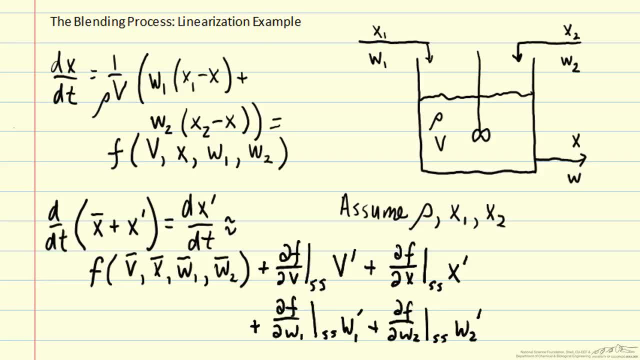 we are evaluating at the steady state value And those are going to be constant values. So the only time-varying quantities in this new model are going to be associated with the deviation variables And those all enter linearly. So the reason that this model is going to be linear is because we're using only a first-order Taylor series approximation. 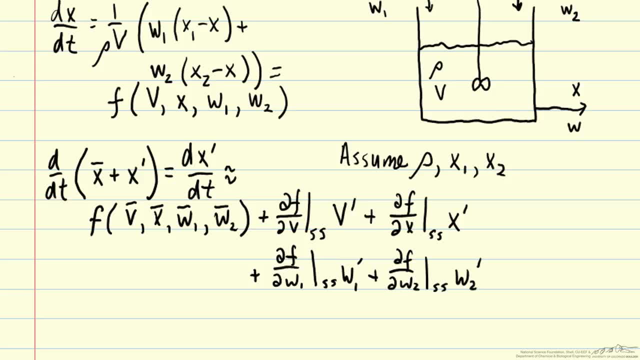 If we wanted it to be more accurate, we could include higher-order terms, but then we would be back to having a nonlinear model. Now let's go ahead and plug in our function f and its derivatives into this approximate linear model. First, we need to evaluate this function at its steady state value. 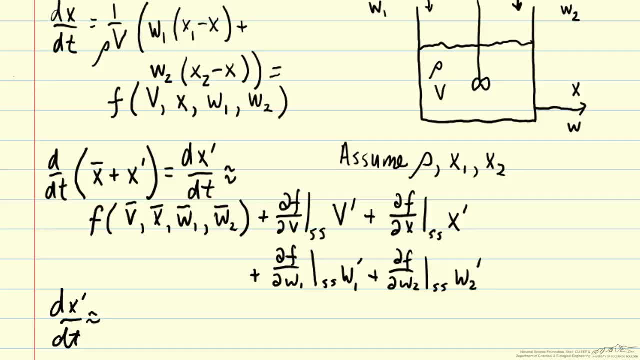 But the function is just the time derivative And at its steady state we can plug in 0, dx dt equals 0, and the bar variables on the right-hand side, And so this term is always going to be 0 for any linearization around steady state. 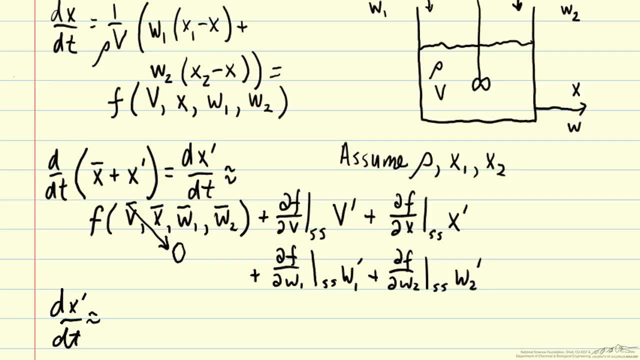 So that's very convenient. We can always cross off that term as long as we're linearizing around steady state. But we do need to go ahead and evaluate these derivatives Now. the first derivative is going to be the messiest because we have 1 over v. 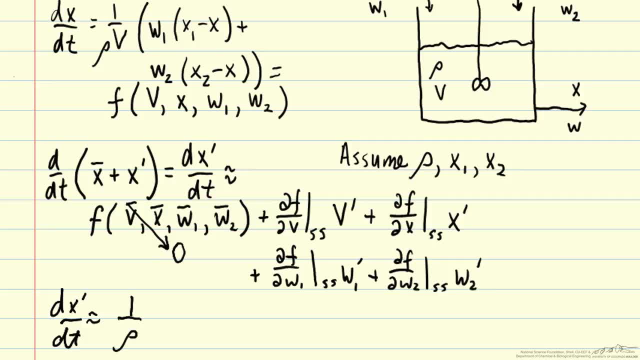 In our differential equation, we'll go ahead and evaluate the derivative of f with respect to v at steady state. So we're basically just going to rewrite all these other terms that we're going to hold at their constant value for this derivative, And then we're going to need to take the derivative of 1 over v. 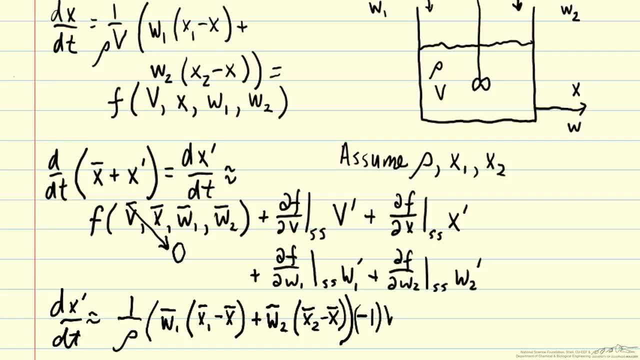 So we're going to get minus 1 v to the minus 2, and we're going to evaluate that again. It's a bar value, And then we're going to multiply this entire derivative df dv by v prime. So that is our first term. 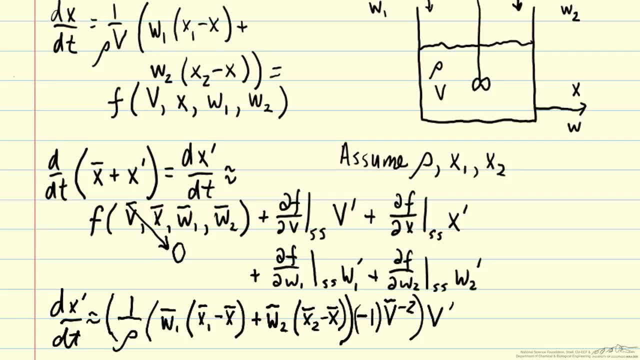 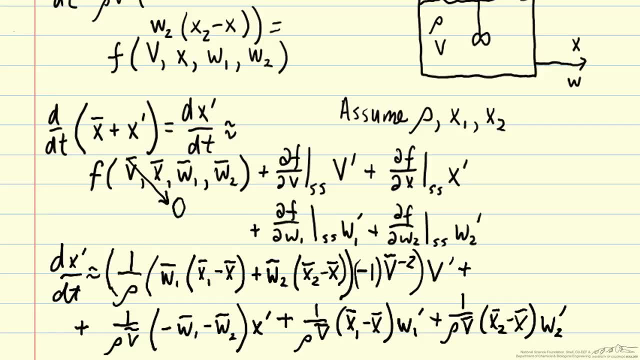 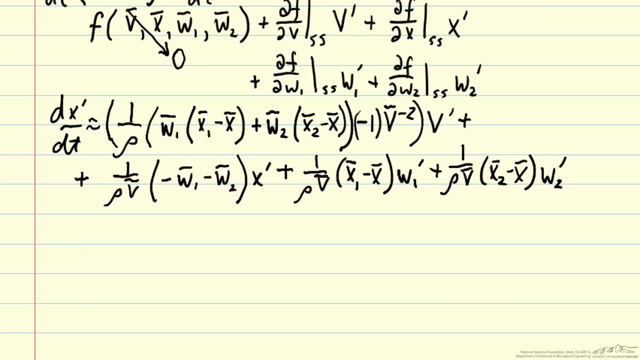 We need to do that three more times, But fortunately the function is not as complicated in order to do that. So that is the linearization for any arbitrary steady state of the system. But let's plug in some numbers, So we'll use the same value. 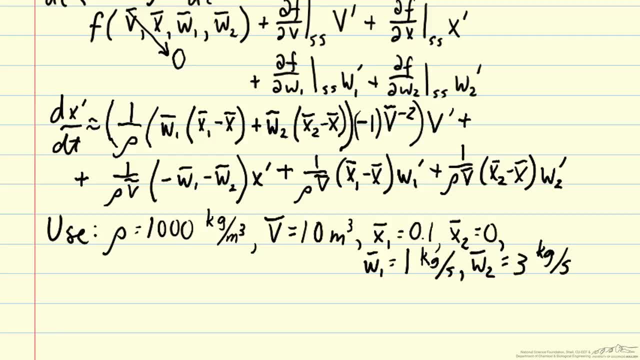 So we'll use the same values that we had used previously, And from these steady state inlet conditions we can then calculate the steady state outlet conditions. So w bar is just the sum of the two inlet streams, So that's 4 kilograms per second. 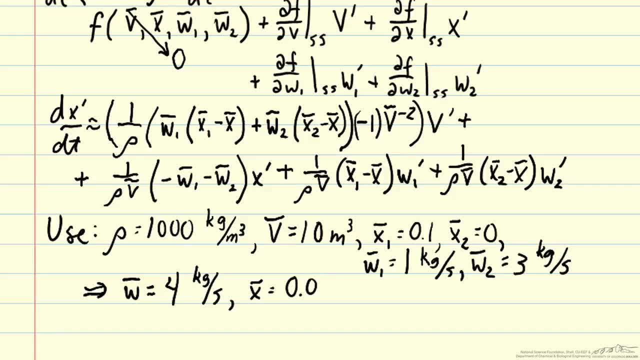